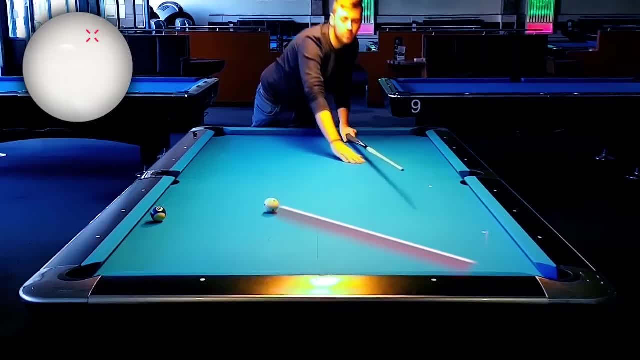 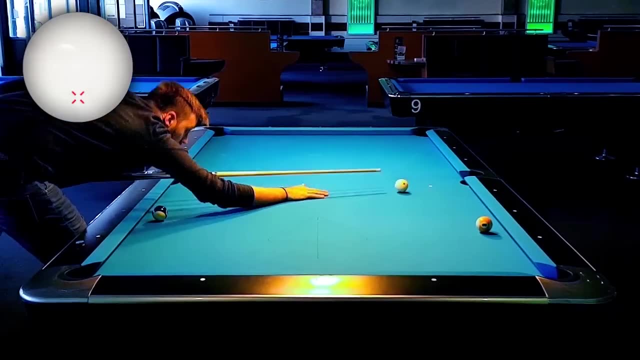 So I'm a long way in the danger zone where I don't have a shot except for a bang, And, as you see, I'm going towards the side pocket again. So let's just avoid it and give ourselves a little bigger angle. Now I can just use the natural path of the cueball. 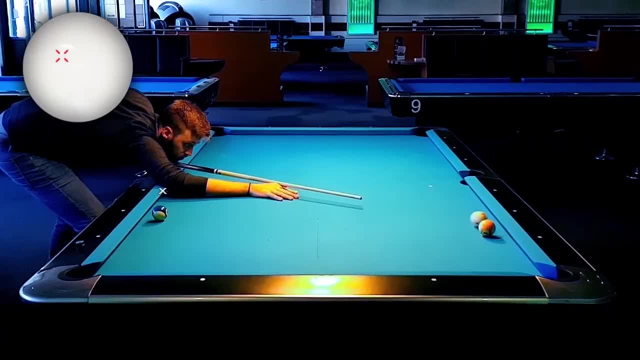 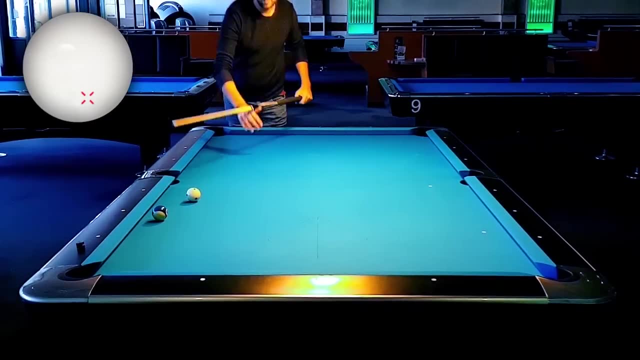 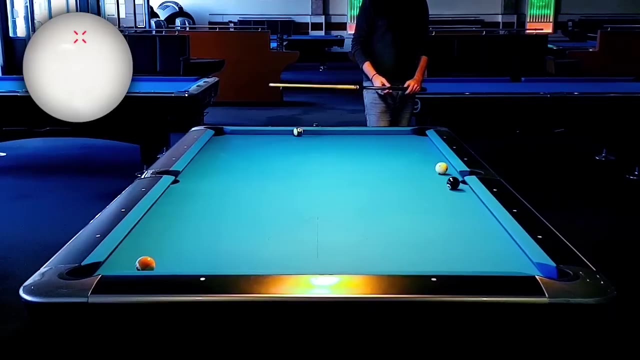 manipulate it a little bit with left hand side and go to the exact point on the rail. So, as you see, I'm just having way more control over the cueball because I don't have to force anything. In our next example we have this situation: 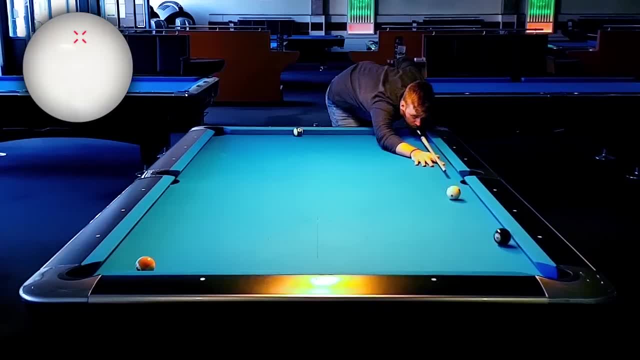 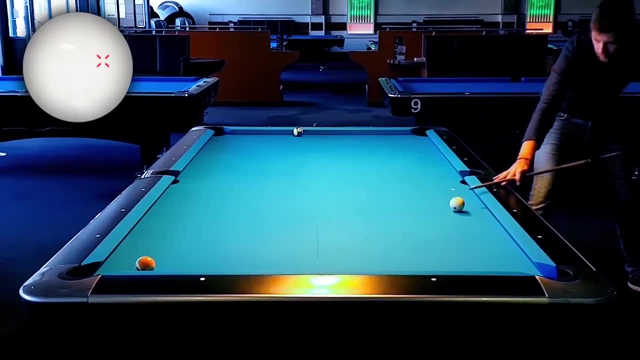 And what beginners would do here is to just follow a little bit so that the shot on the 9 gets easier. But what happens here is I have to force the cueball again to go up table and hit it really hard, because I'm hitting the 9 ball very full. 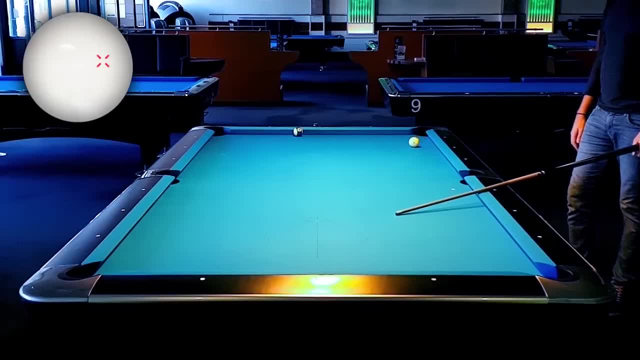 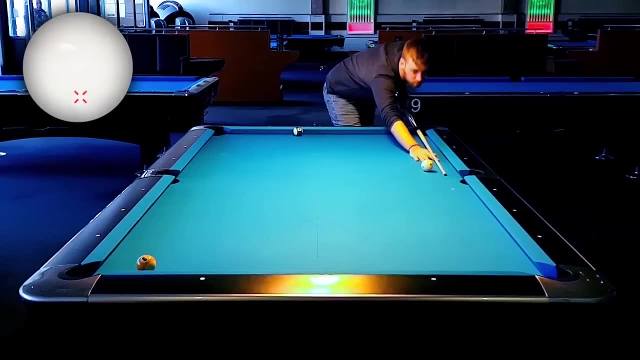 And because of that I over hit the ball, So I'm deciding to draw the cueball back. I'm now further away from the 9 ball, but since the 9 ball is hanging over the pocket, the putt is not that tough. 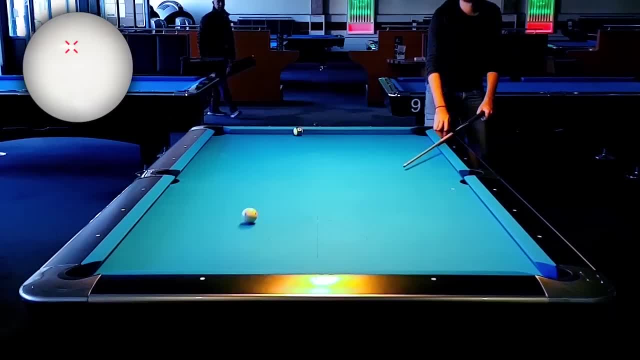 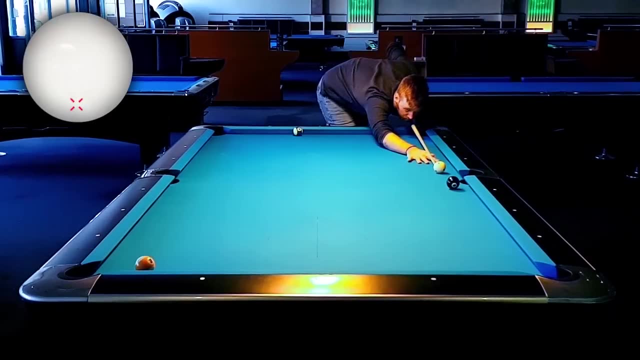 Now it's much easier to go up table. But you see I got too short, So now a short excursion. When I'm playing the 9 ball I use the short rail to get position, Because then my margin for error is just smaller. 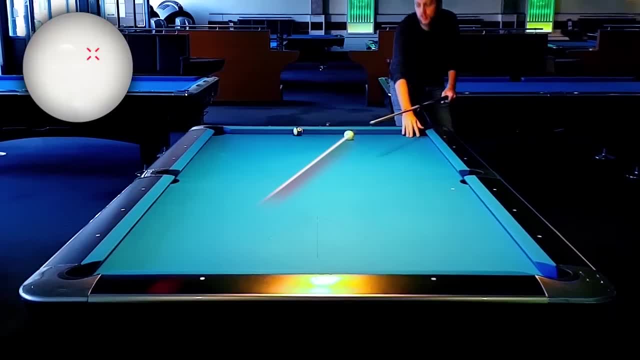 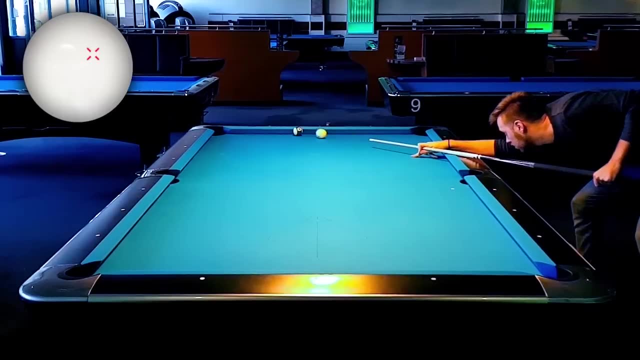 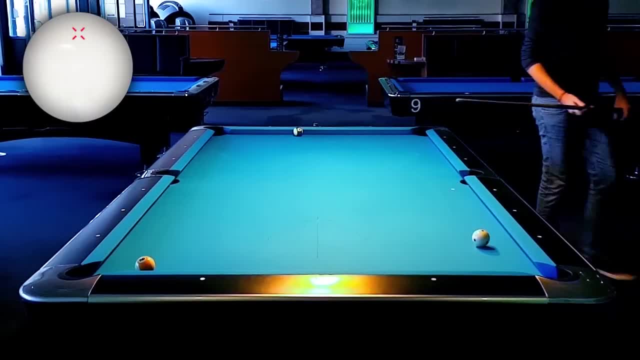 And the cueball is just a nice and easy position to do. Just follow the cue ball and avoid the scratch. And here again you want a big angle on the 9 ball so that you can go up table with a little bit of supporting right hand side. 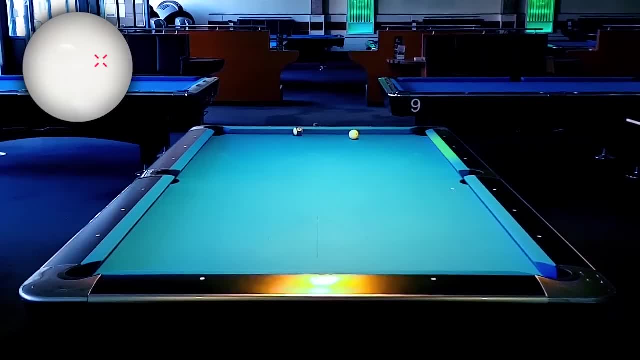 Hit the second rail and get a nice and very easy position for the 10 ball. In this example I also have a little bit of support, But you can also do a little more support. But if you want to do a little more support, you can go up table. 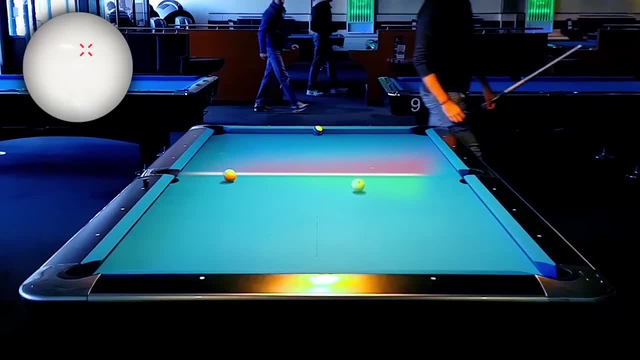 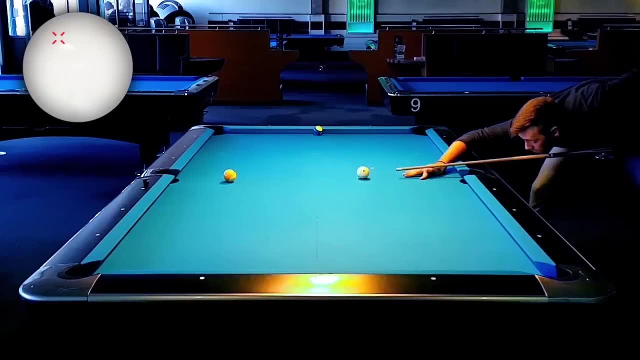 want to get on the right side of the nine, of course, and again, I play for the bigger angle, because if I play for that slight angle on the nine, I have to risk to come too short and have to go the long way all around the table and as you. 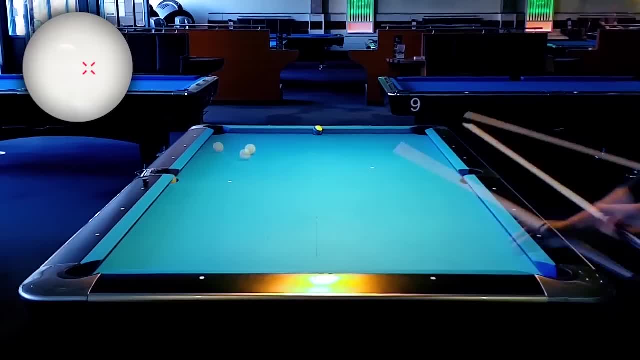 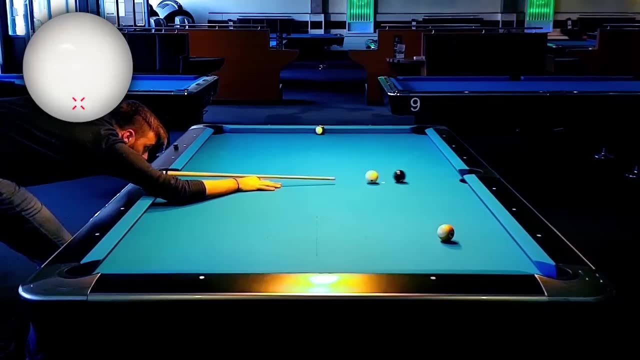 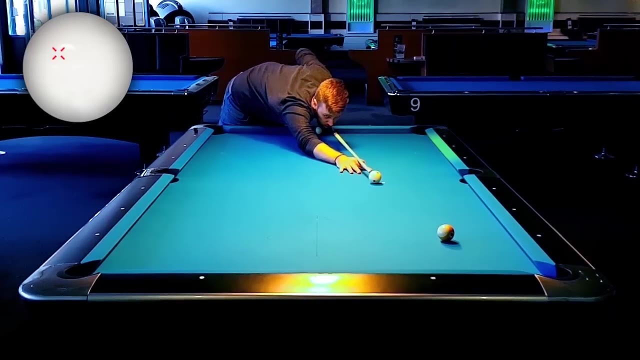 see. even a bigger angle poses no problem. I can just play the same shot and roll the cue ball in. this example is similar to the first situation. I just play a stop shot and have to force the cue ball up table. see what happens when I just follow the cue ball a little more. 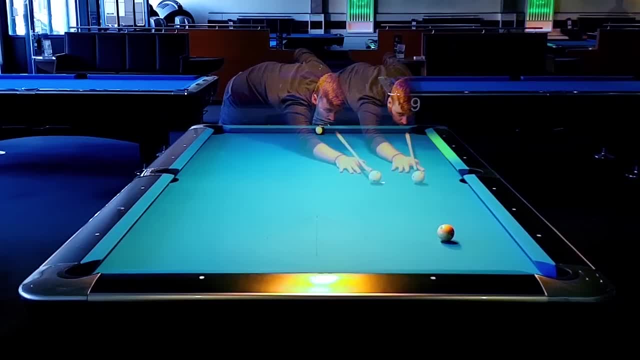 do you see the difference in my strokes? I? I didn't have to work hard on the right side, where I had the bigger angle on the nine ball. on the left side, you see how hard I had to hit and I how I had to force the cue ball. both ways are possible, of course, but we want to make 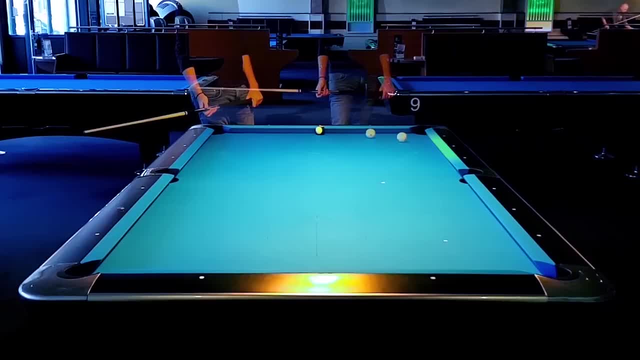 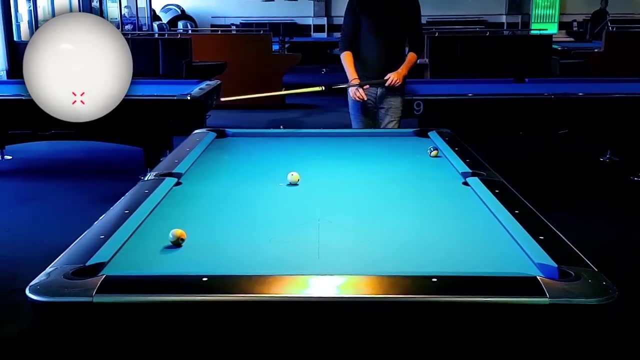 it as easy as possible to get position for the next ball, and that's obviously easier with more angle on the nine ball. same here: I just play a stop shot and have to force the cue ball and play a draw shot. but this is dangerous because I have to use the right side of the ball and the right side of the ball to get. 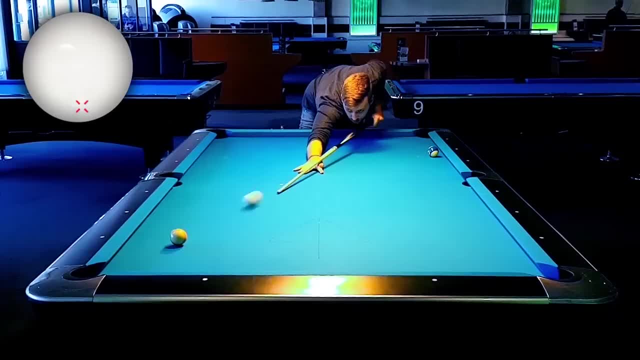 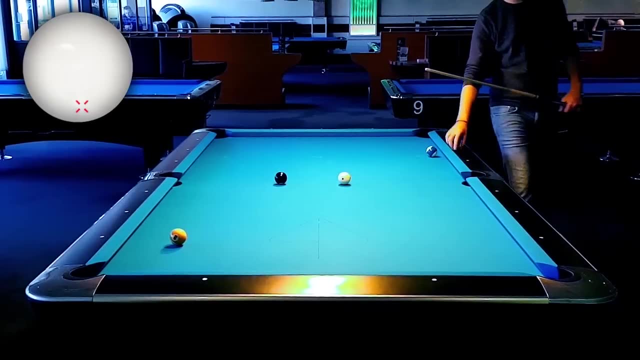 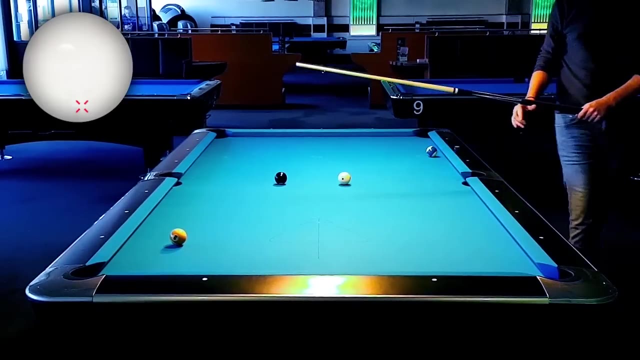 the right side of the pocket to create an angle and that way I can easily miss. so on all these shots, we should have learned one very important lesson: step behind the nine ball and look what angle you want to have from there. I'm seeing a stop shot is very bad choice, so I decide to draw the cue ball back to have a nice. 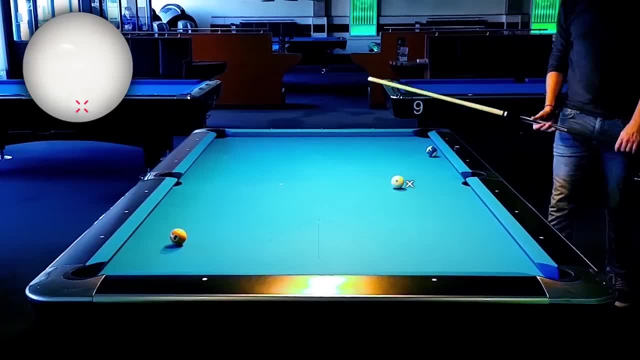 angle on the nine ball, but I don't agree 100% with that shot. you see, I overrun the position and get a nice angle on the nine ball, but I don't agree 100% with that shot. you see, I overrun the position and get a. 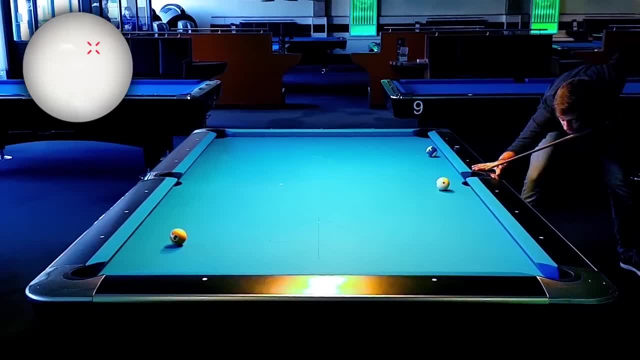 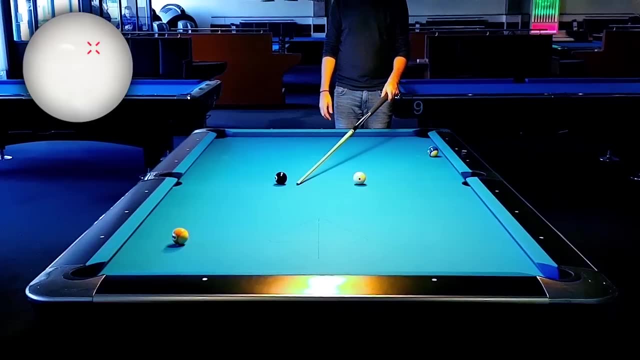 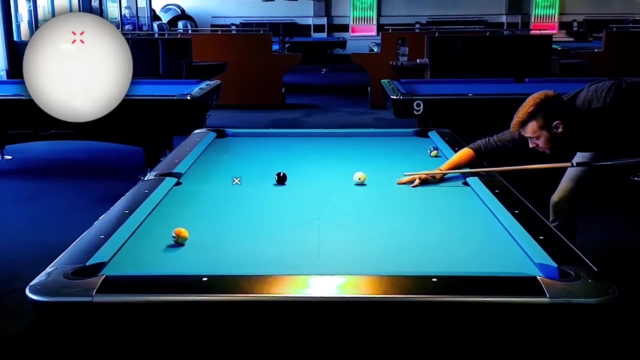 and get a tougher shot on the nine ball that it should have been so again I'm stepping behind a nine ball and see that this angle on and nine ball is perfect to get easily to the temple. I have to be a little careful because I'm flirting. 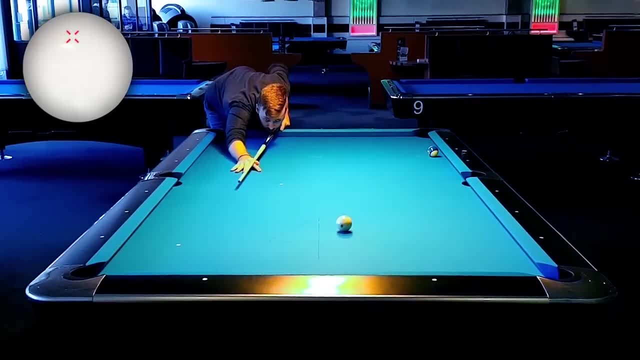 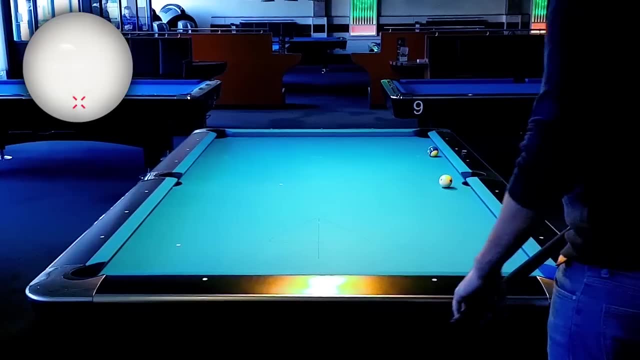 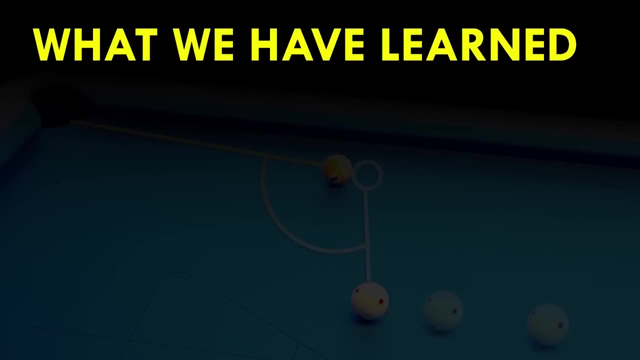 with the side pocket. but to prevent it, I played the shot soft enough that the cue ball would get too far, so that the cue ball will never reach the side pocket, even if the line is going exactly towards it. so what have we learned in this lesson? the right angle makes it easier to go to the next ball. 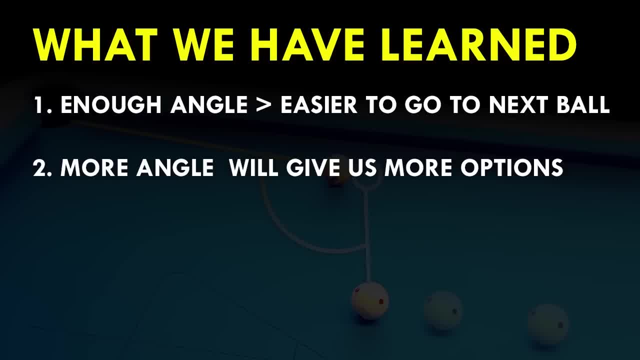 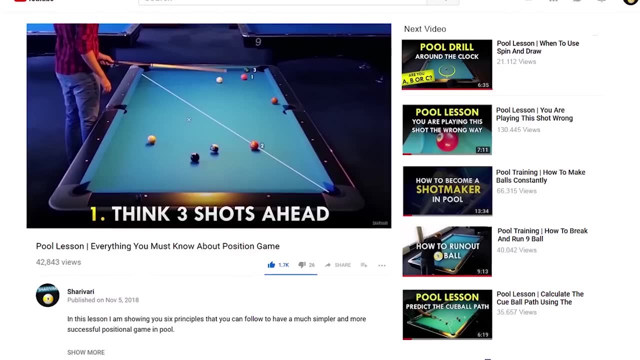 more angle- not too much, of course- will give us more options. the less angle, the less places we can go with the cue ball and step behind the next ball and think where you want to be for the next ball. that's the free ball. i had principle from my video: everything you have to know about positional 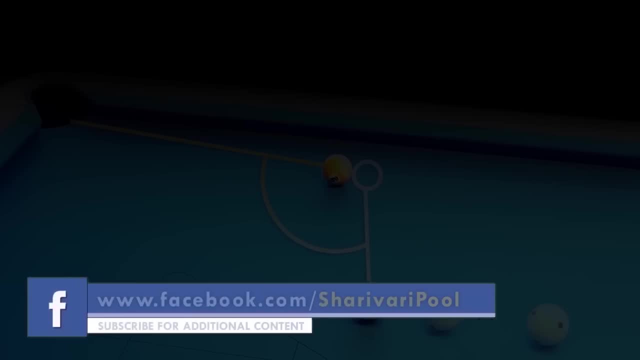 play. well, i know not everyone likes angles in a ball because it makes the shot, of course, harder. but if you not have enough angle and have to force something to get to the next ball, the shot also becomes harder. so you have to train these angles. that shot would be much harder to get from the shot to the ball. 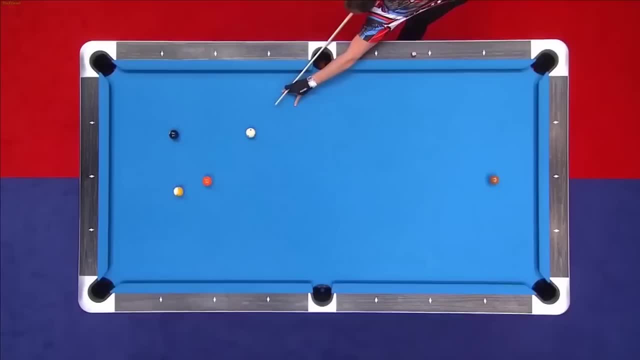 with angle. do not pose a problem for you anymore. 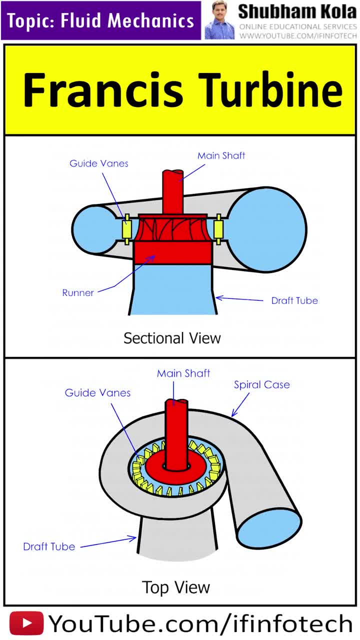 Construction and working of Francis turbine. This turbine is a combination of Impulse and Reaction turbine. Francis turbine consists of spiral casing which is inlet medium of water to turbine, where water flowing from reservoir is made to pass through pipe with high pressure. Here blades are circularly placed. where water striking, the blade should flow in circular axis. 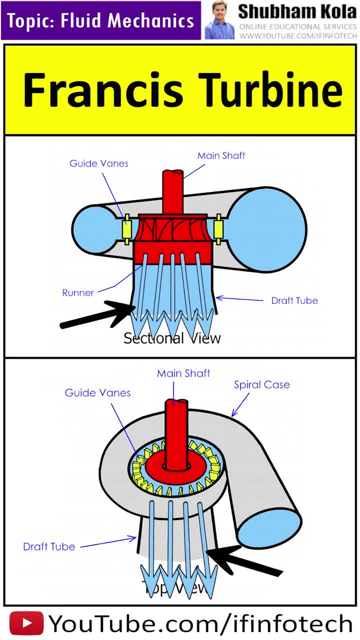 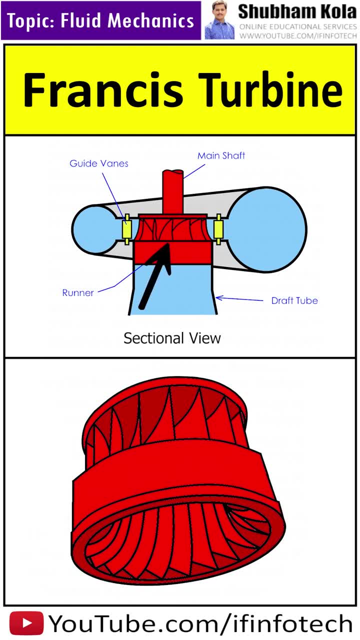 Here pipe of gradually increasing area is used for discharging water to tail race. The pipe of increasing area is called as duct tube In Francis. turbine runner blades are divided into two parts, where lower half part is made in shape of small bucket, where impulse action of water is used to rotate turbine. 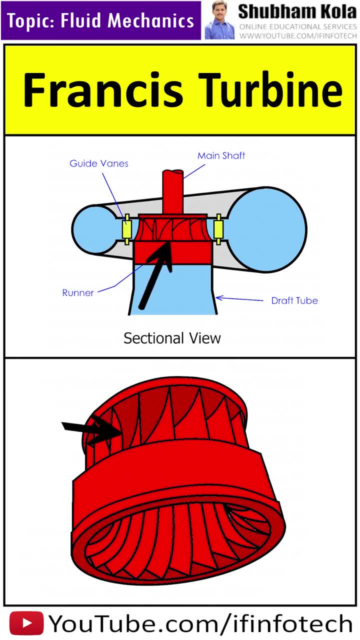 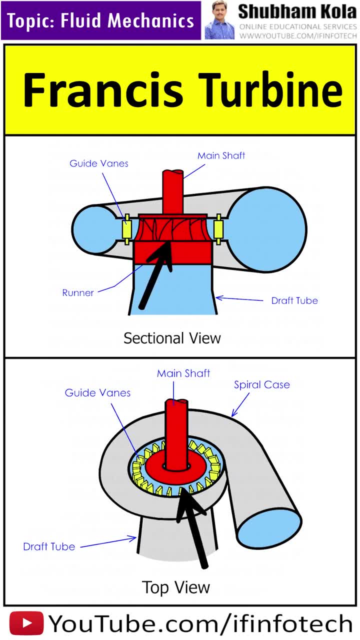 and upper part of blades use the reaction force of water flowing through it. These two forces together makes the runner to rotate. The runner may be keyed to shaft, Hence shaft rotate, and we got mechanical work. and then, with the help of generator, the electricity is obtained.